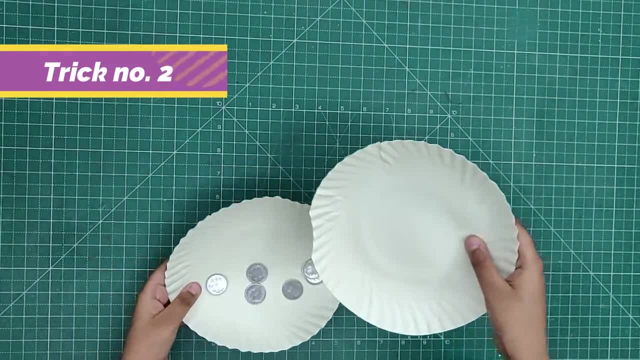 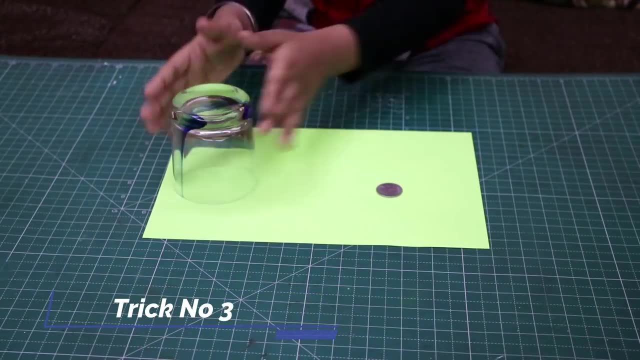 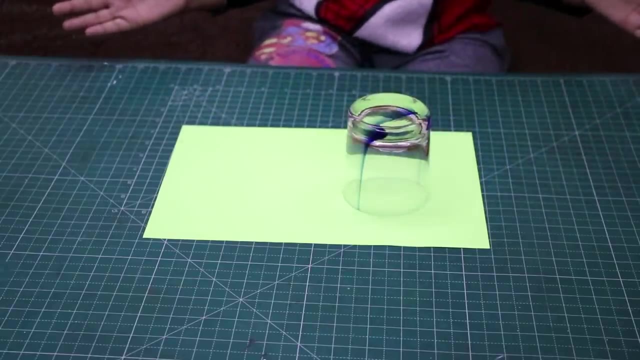 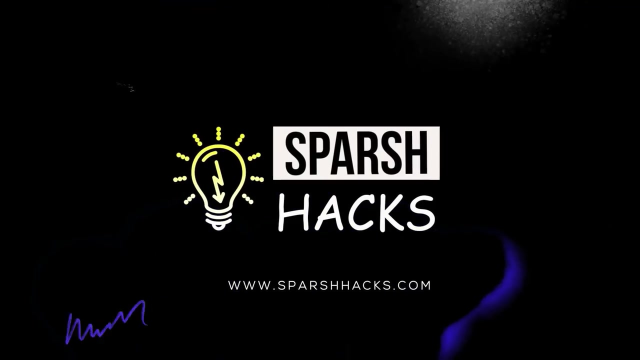 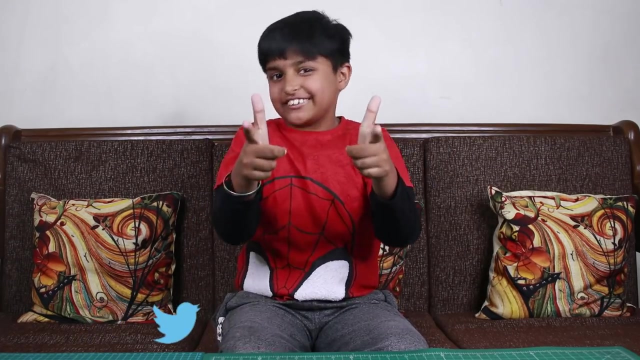 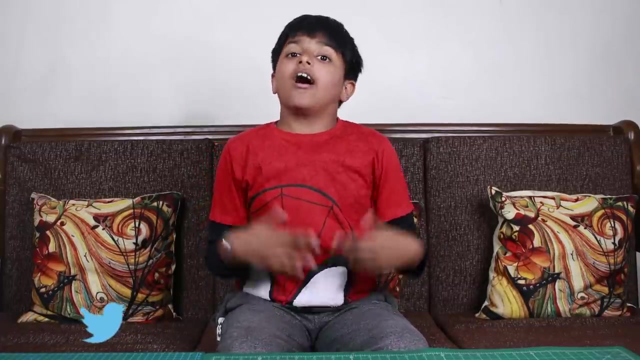 Let's see the magic. Three, two, one. What From three coins? now there are six coins. You see this coin and you see this glass. Now this coin will disappear. Oh, it vanished Here in the cards and in the description box. 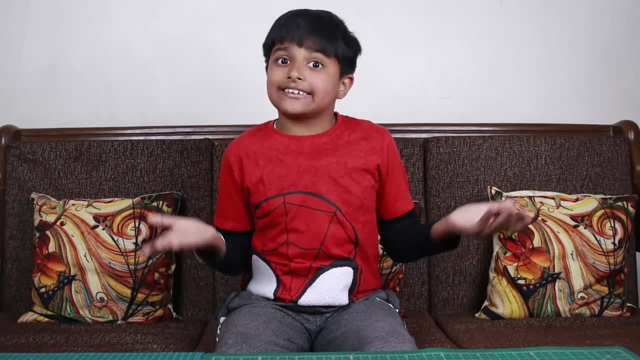 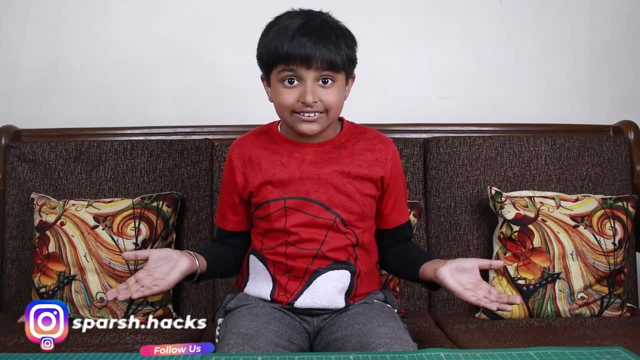 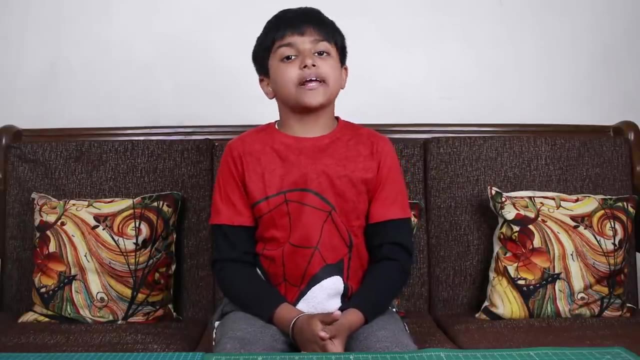 So in today's video we will do three more very simple magic tricks. You can use these magic tricks to amaze your friends, So let's see how to do these magic tricks. Before starting the video: if you have not subscribed to my channel, then subscribe and click the bell icon. 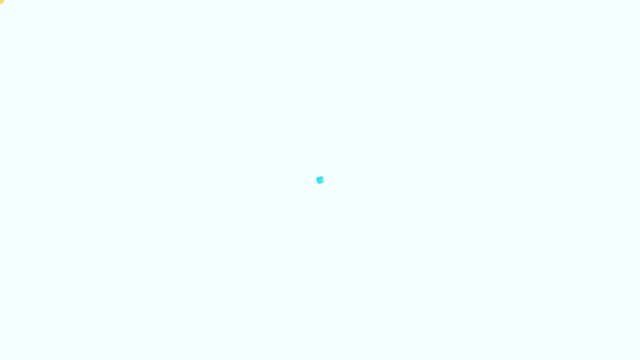 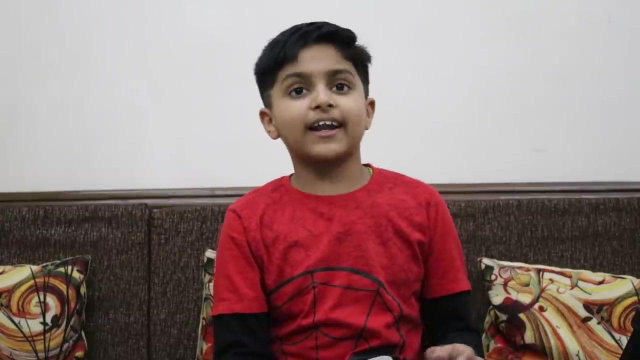 So that you get updates of my new videos. And if you are new here, then subscribe to my channel And then you will get regular updates of my videos. Our first trick is the disappearing stick. Abracadabra, ghillie, ghillie, choo. 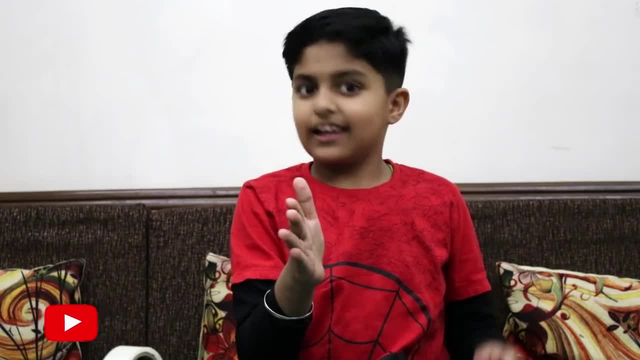 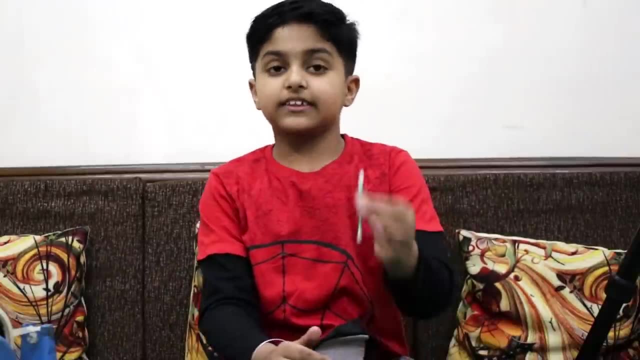 Oh, where did it go? Let's bring it back. Abracadabra, ghillie, ghillie choo. Oh, it's right here. I have taken an ear bud for this. You can take a toothpick if you want. 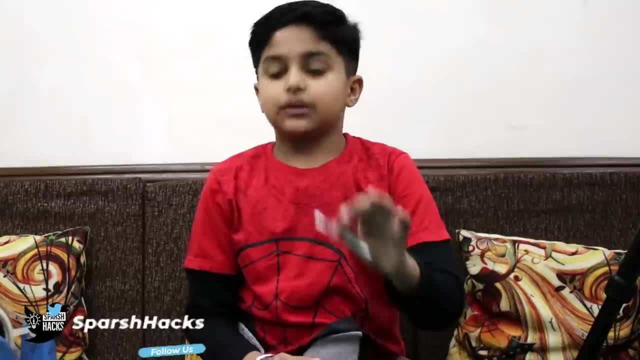 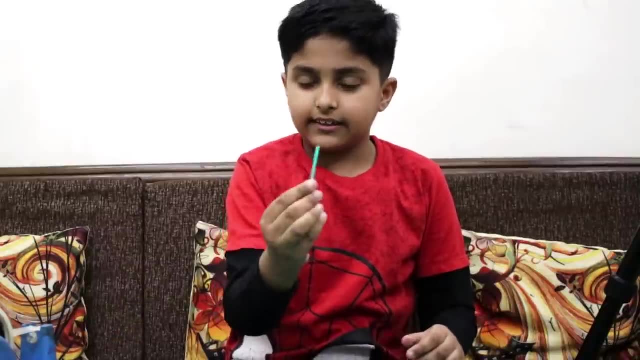 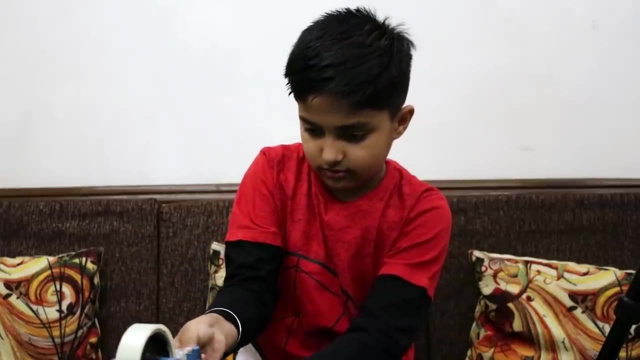 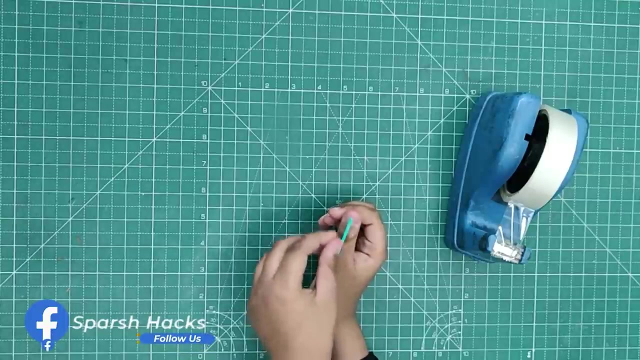 You can take a toothpick if you want. So first of all, So, first of all. So, first of all, We will cut it a little bit. so I have cut it in half. now I will paste it on my thumb with cello tape. you have to put the tape right here in the corner and paste it right here so that it does not go in front of your thumb and does not show from here. 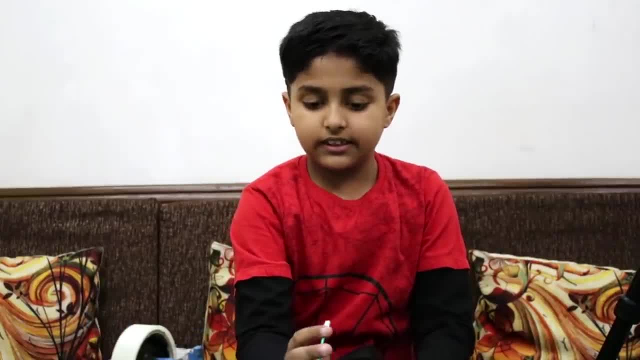 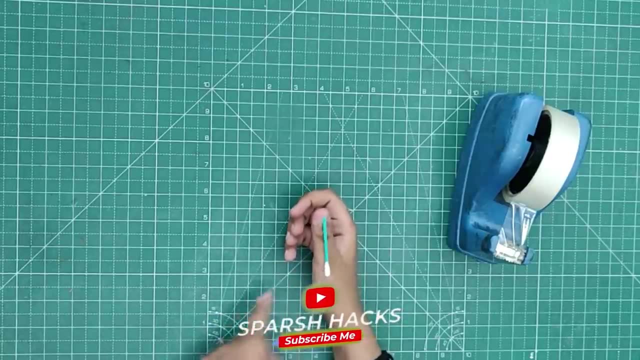 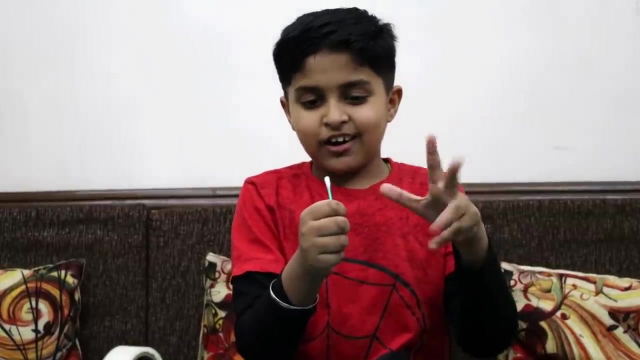 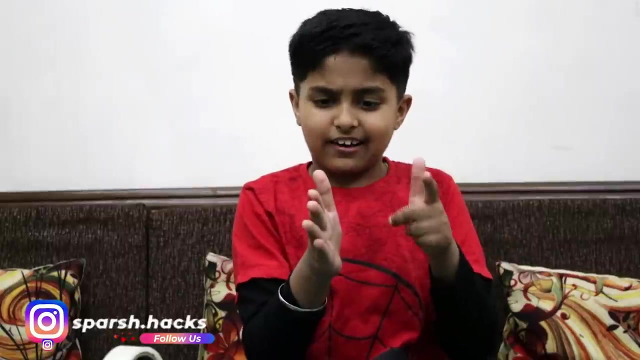 See, when I am bending it, it is coming up like this, and when I am straightening it, it is straightening. now let's see the magic: abracadabra ghillie ghillie choo. oh, where did it go? let's bring it back. abracadabra ghillie ghillie choo- oh, it is right here. 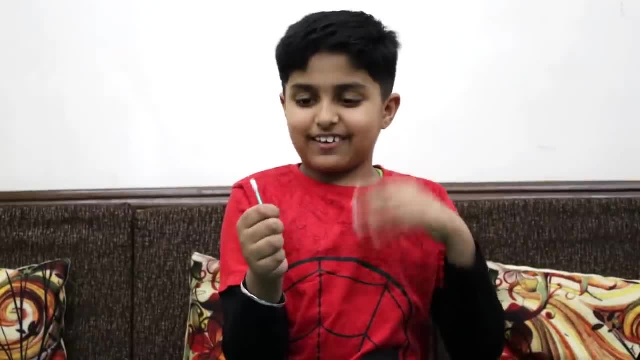 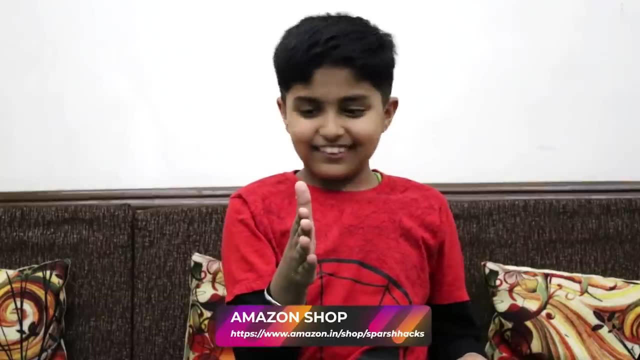 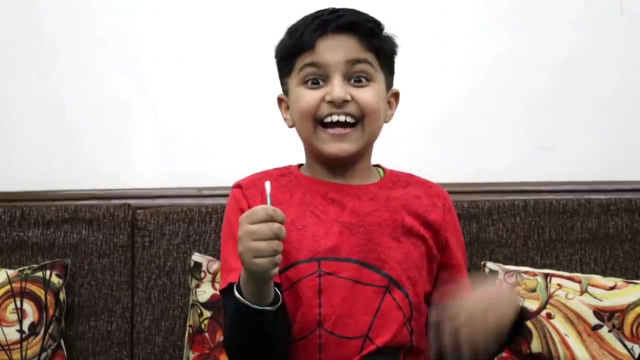 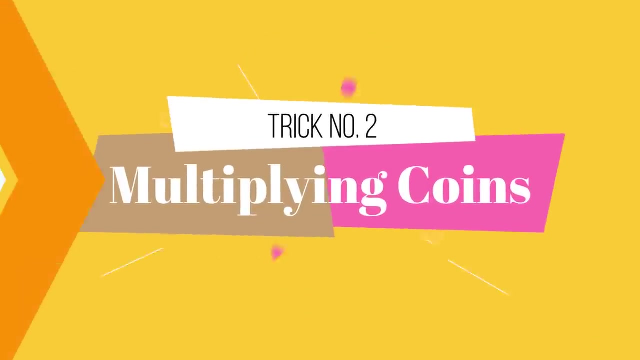 Let's try it again. abracadabra, ghillie, ghillie choo. oh, where did it go? let's bring it back. abracadabra, ghillie, ghillie choo. oh it is back again. this trick's name is multiplying coins. now you have learnt three coins. 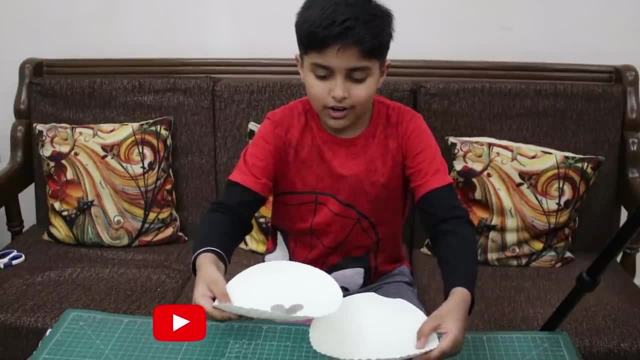 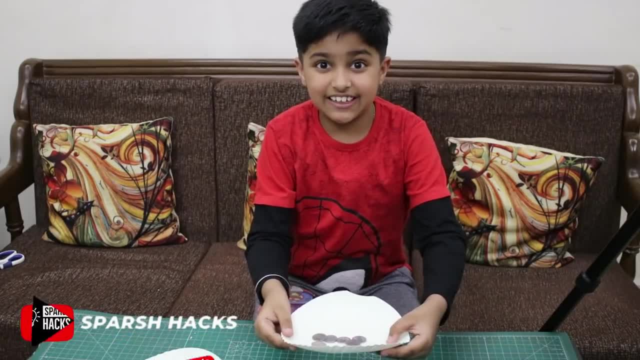 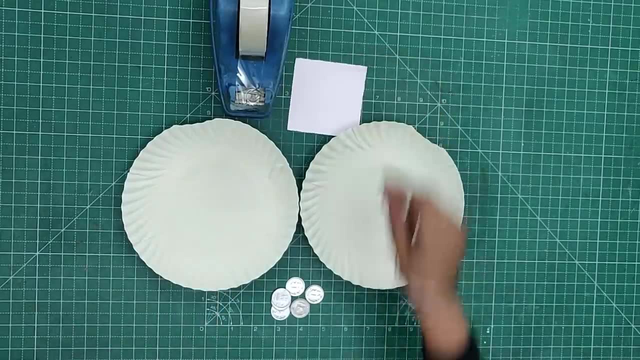 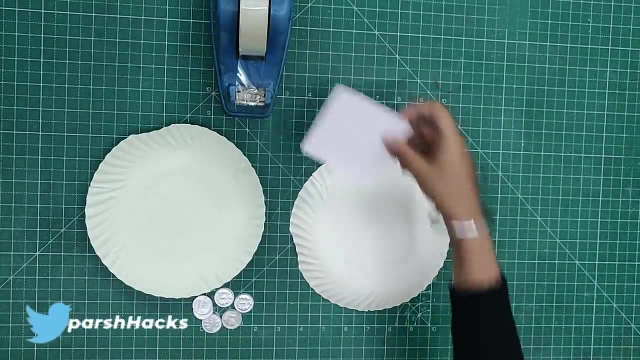 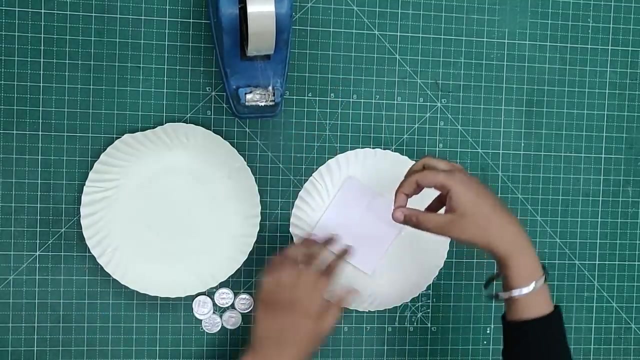 Let's try it again: abracadabra, ghillie, ghillie, choo. oh, it is right. here Now there are six coins magic. For this trick we need two paper plates, a piece of paper and few coins. So first I will take one paper plate and I will paste the paper here. 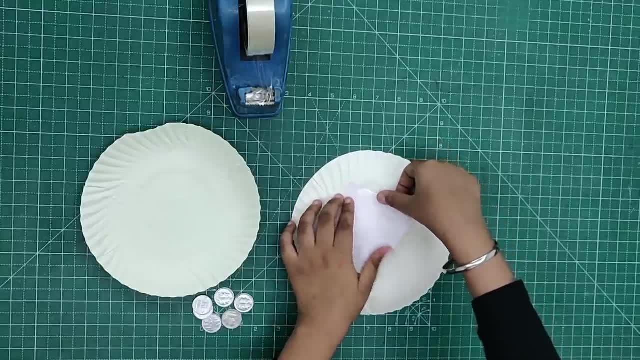 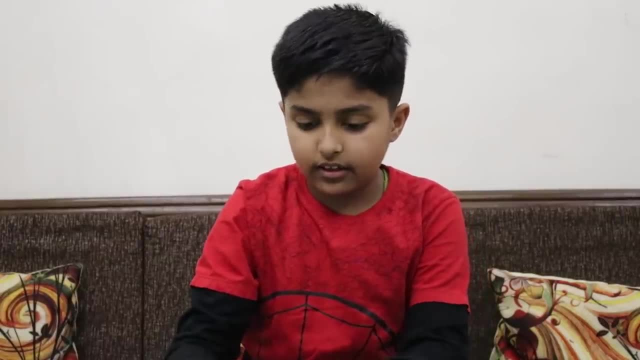 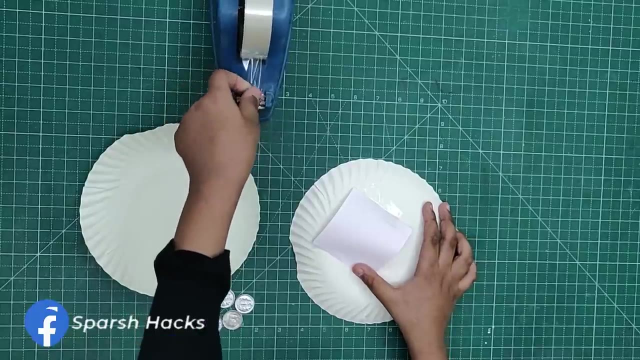 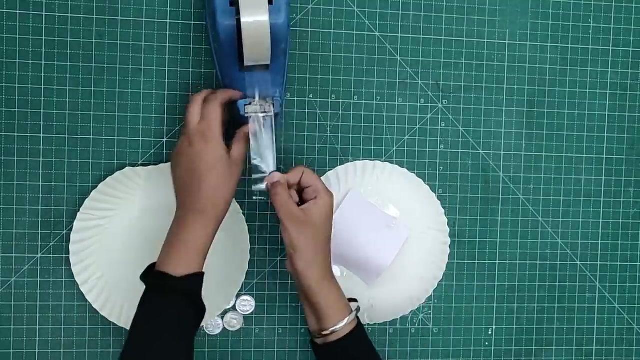 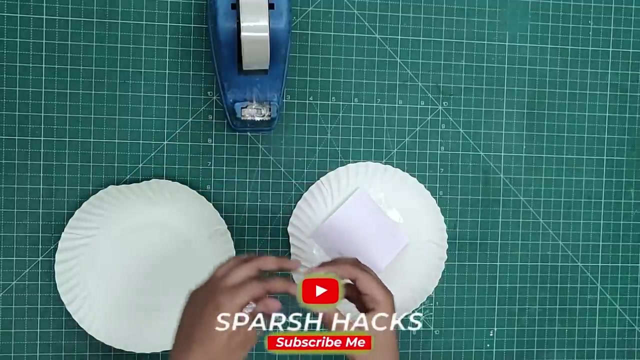 So first I will take one paper plate and I will paste the paper here. Then I will take the other paper plate and I will paste it from this side. Then I will take the other paper plate and I will paste it from this side. Now I will paste this side as well. 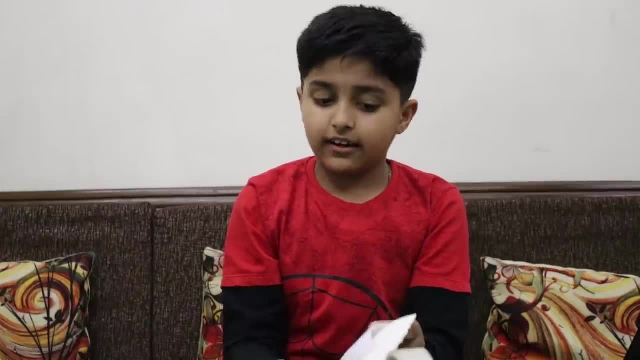 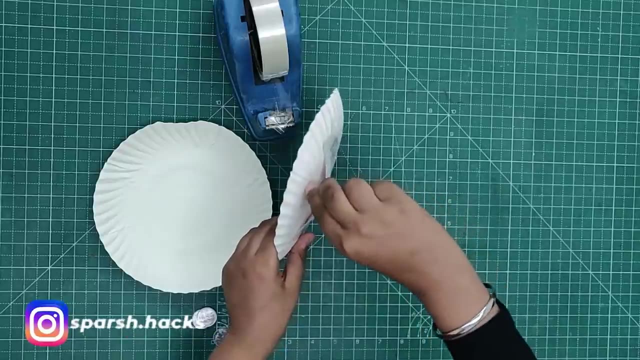 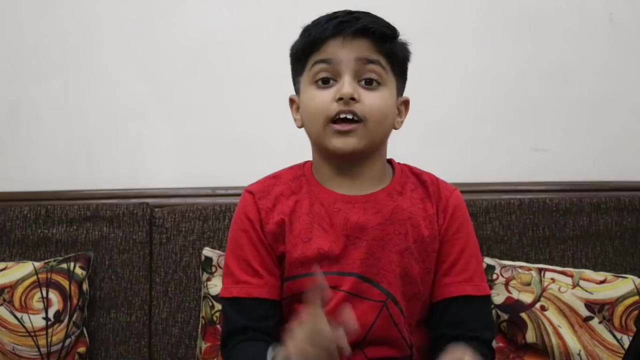 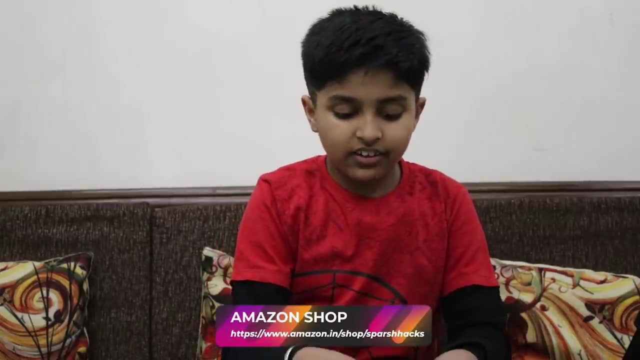 So this is one pocket. You have to make sure that it is completely sealed So that the coins come out. So I am putting 3 coins inside this. Now let's see the trick. How does it work? So, for the trick, I have put 3 coins inside the pocket. 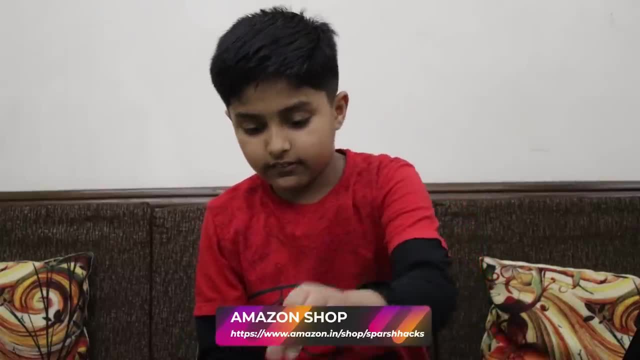 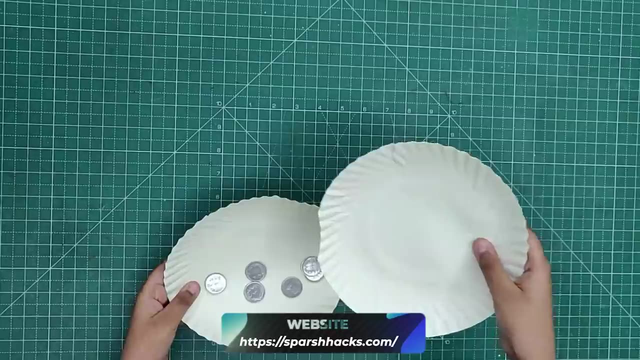 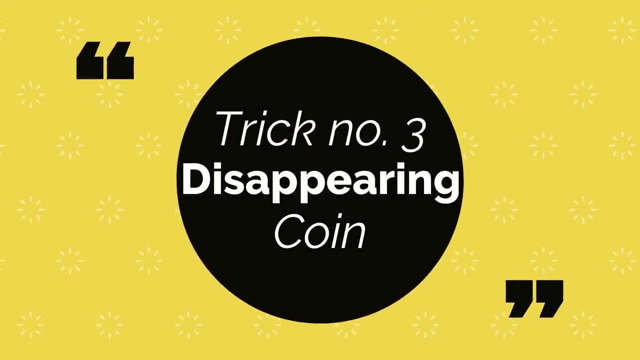 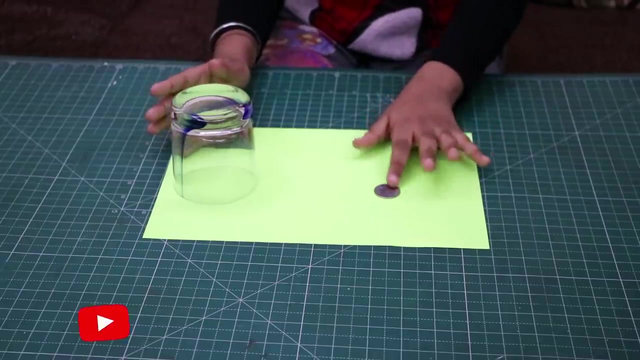 And now I will put 3 coins inside this. Let's see the magic: 3,, 2, 1 From 3 coins, now there are 6 coins. This trick is called the disappearing coin. You see this coin And you see this coin, This glass. 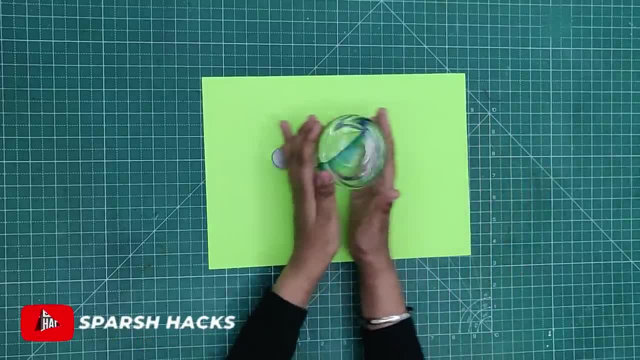 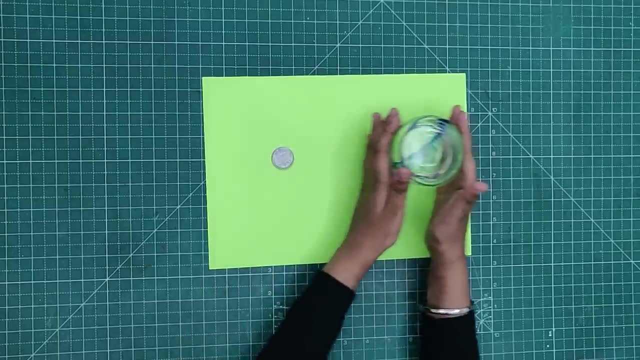 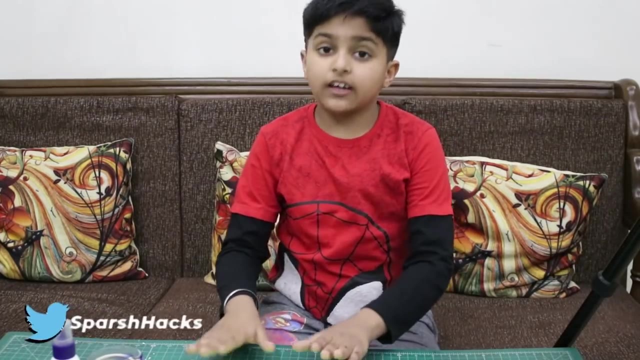 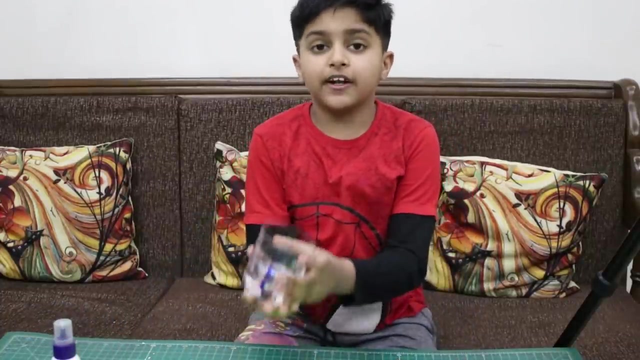 Now this coin will disappear. Oh, it vanished. Now let's bring it back. Oh, it's back again. For this trick, we need a big colored paper And a small piece of the same color, And we have taken this transparent glass. We will put a call on it as well. 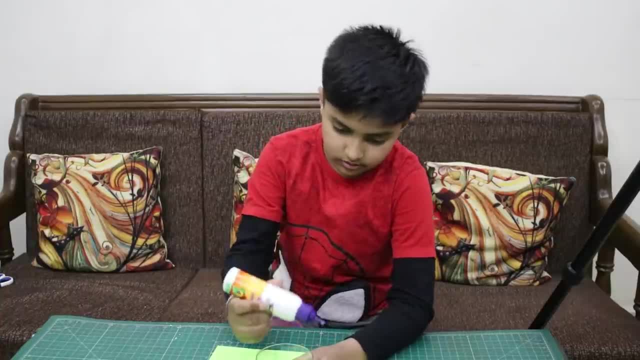 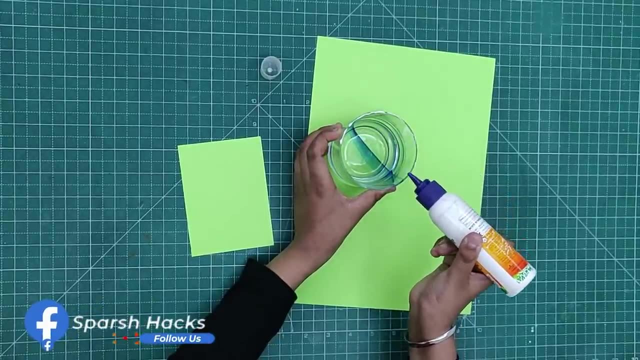 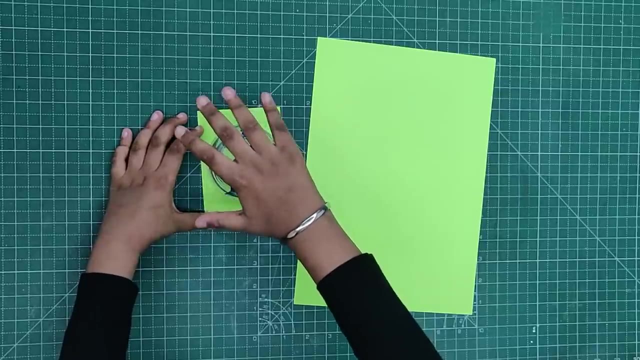 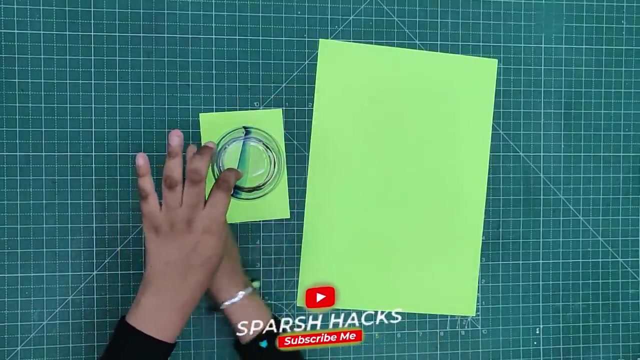 Here is thecker. Hmmmm, And let's see what we get: The scammerrod. I have collected all the coins And did you know? I've got the coin. Yes, I've got the coin. I saw this coin at the station. What's this? 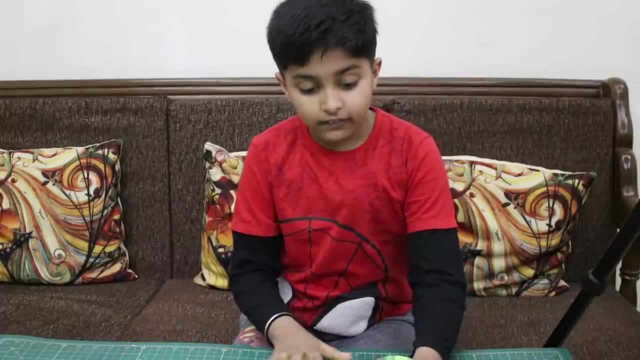 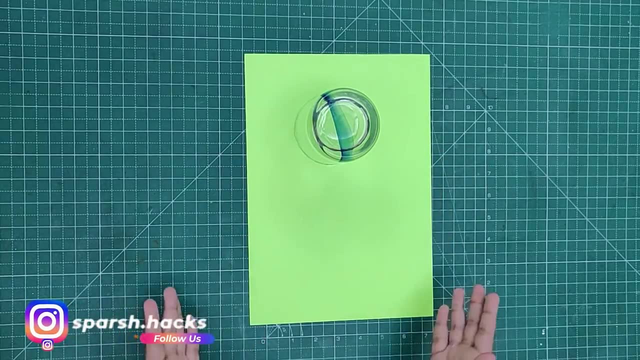 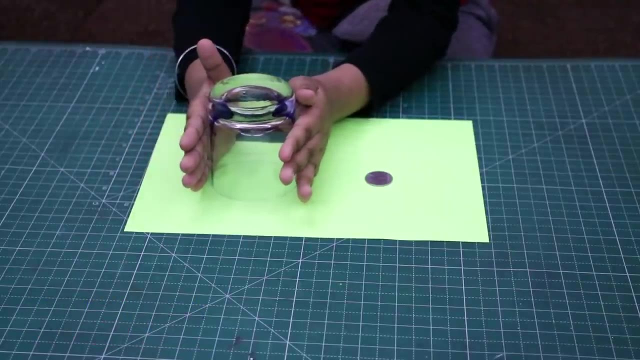 Friends, look, if we place the glass on the paper, then we don't even know that there is a paper of the same color under the glass. Now, let's do the trick. We will hold this glass like this and move it like this. 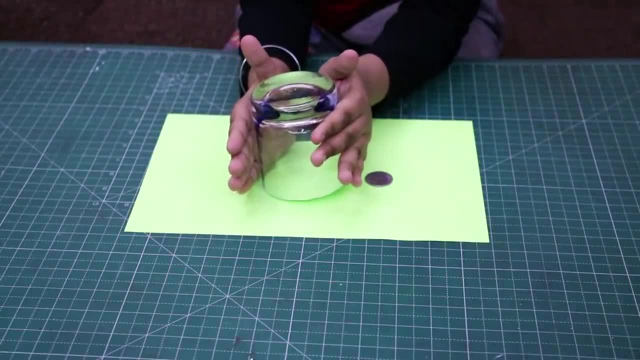 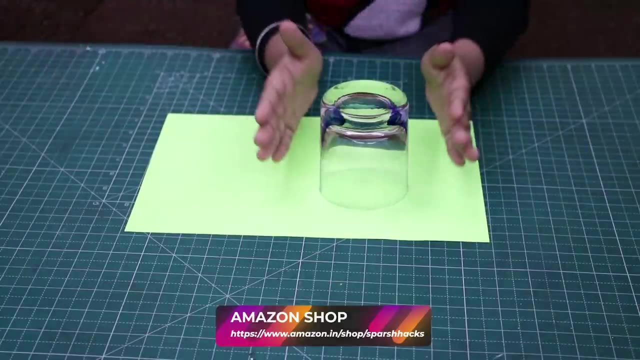 So when we reach near the coin, we will lift it a little up. Then, moving forward and the coin is covered, It vanished And to bring it back we will lift it up again, like this: Back, back, back back. 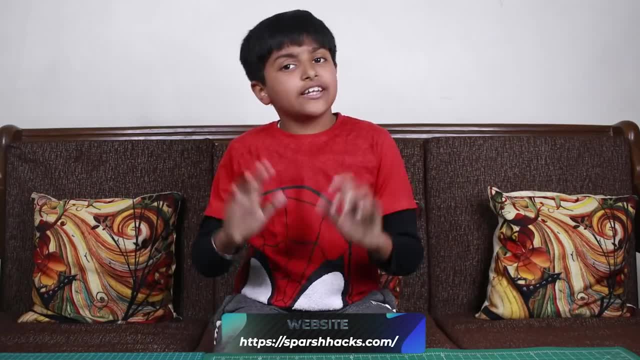 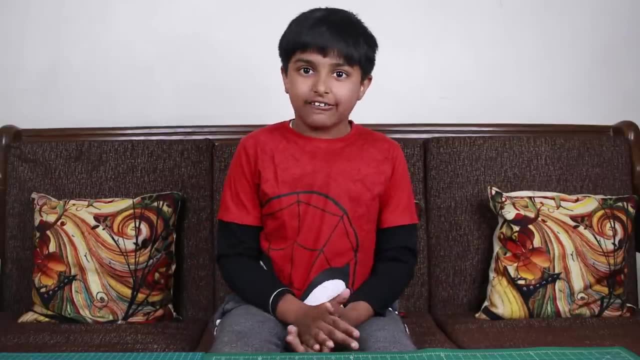 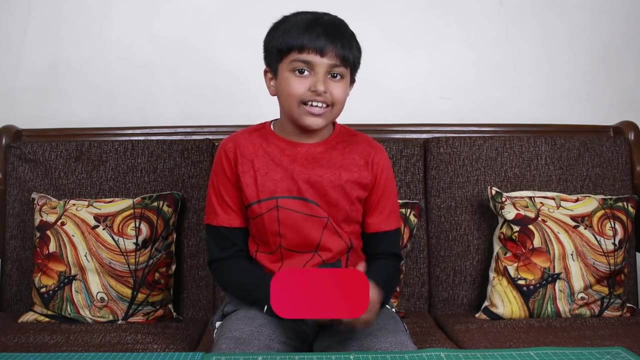 And it's back on the paper. So, friends, weren't these very simple and interesting magic tricks? You also do them and amaze your friends. Do share their videos with me on my Facebook group. If you liked today's video, like, share and subscribe to my channel. 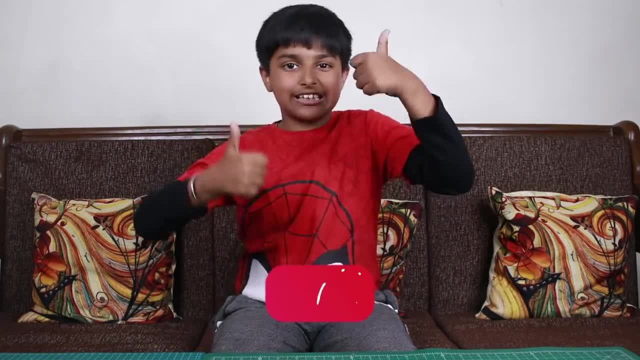 Bye. Have fun with the magic tricks.